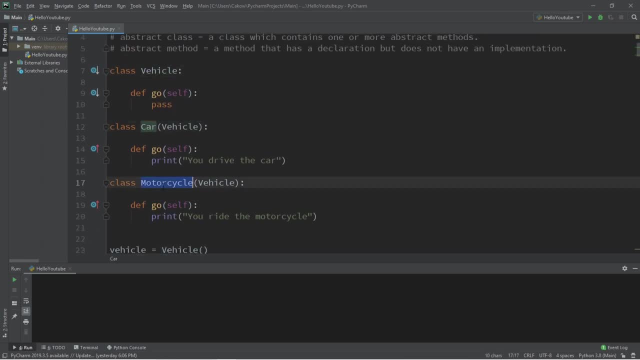 Class: Vehicle, Car and Motorcycle. Car and Motorcycle are the children classes of the Vehicle class. Now, within the vehicle class, there are three classes. Within this vehicle class, we have a Go method, but I'm currently only defining it, not actually implementing it, so I'm just writing pass. 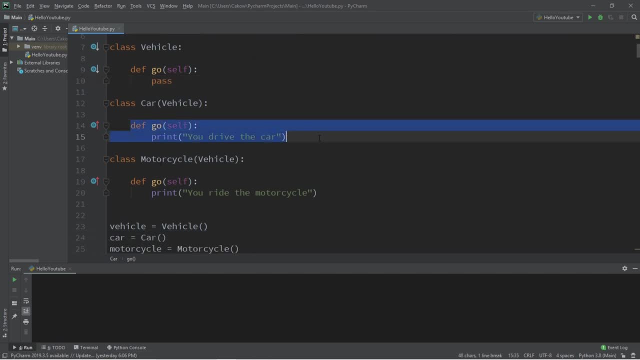 Now, within Car and Motorcycle, we're overriding this method and creating our own implementation of this Go method that we inherit. The Go method for the Car will print you drive the car and the Go method for the Motorcycle class will print you ride the motorcycle. 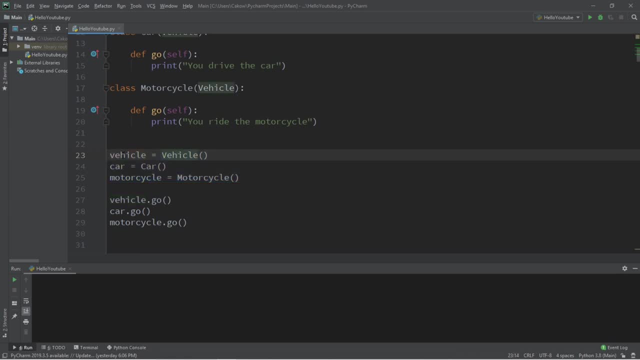 Now, currently I'm creating an object of each of these classes. I have a generic Vehicle object, Car object and Motorcycle object. So after running this program, currently the Go method within our Vehicle class is not being implemented, so this won't print anything. 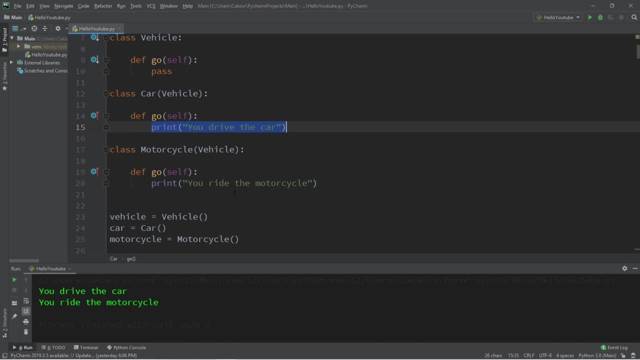 but the Go method within our Car class will print you drive the car and the Go method within our Motorcycle class will print you ride the motorcycle. With that being said, let's pretend that we're coding the next Need for Speed game and we would like a user to create an object from a specific kind of vehicle. 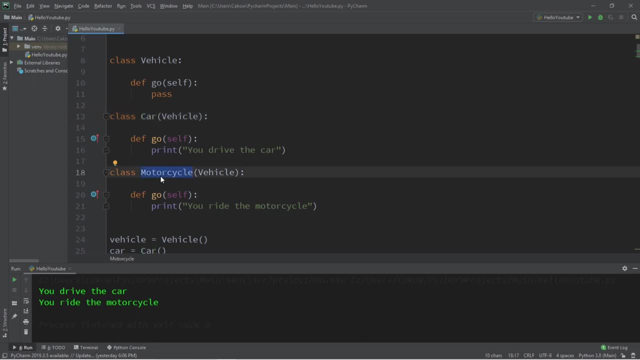 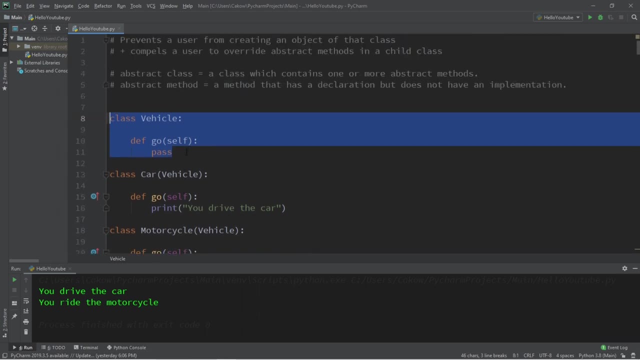 whether it's a car from the Car class or a motorcycle from the Motorcycle class. We would like to prevent a user from creating an object of the Vehicle class because the Vehicle class is too generic. We do not have all of the implementations set up for a vehicle. 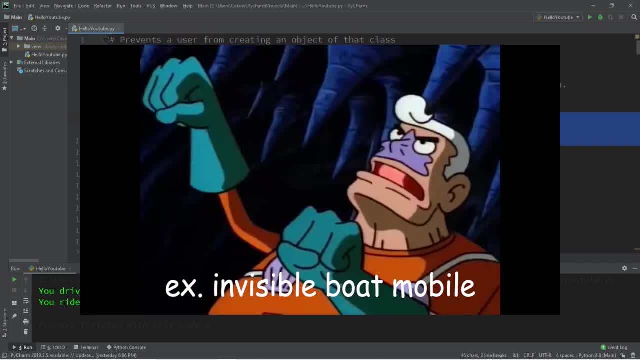 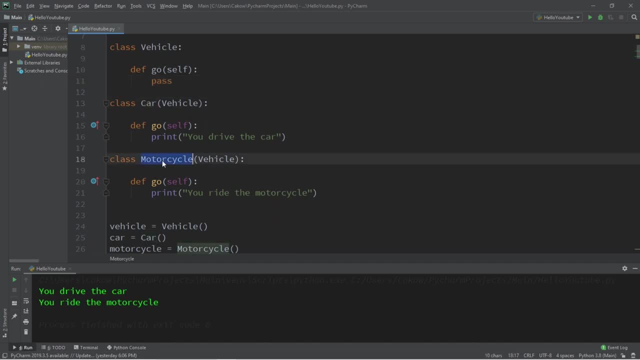 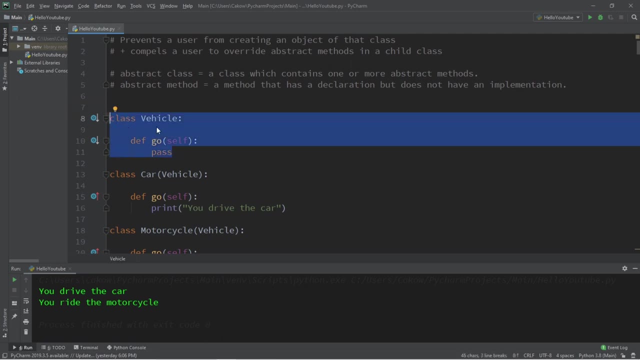 It would be like somebody unlocked the Ghost car or the Invisible car, which doesn't actually exist and is missing a lot of features. We need a user to create an object from a Child class because these are fully fleshed out, And one way in which we can prevent a user from creating an object of this class is well to turn this class into an Abstract class. 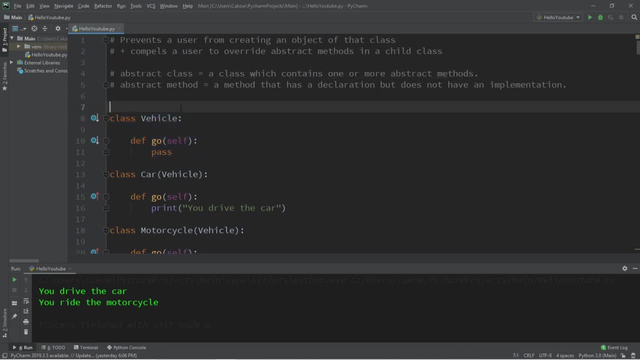 Which is what this video is all about. Go figure Now. the first step to creating an Abstract class is that we'll need some imports. So at the top of your program write this From ABC: ABC is an acronym for Abstract Base Class, ABC. 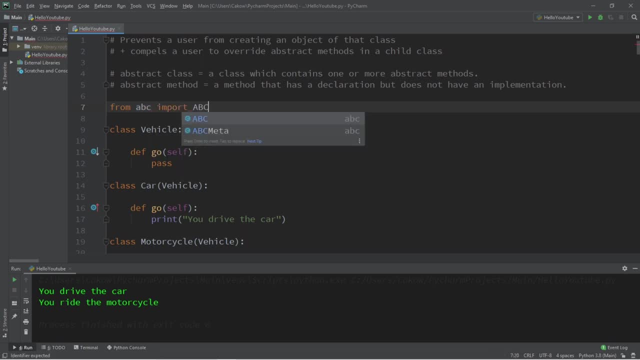 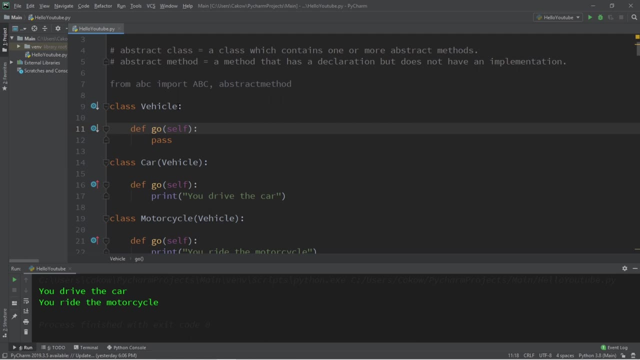 From ABC, import ABC, all capital comma. Abstract Method: Alright, now, with our Vehicle class, the class that you intend to be the Abstract class, add a set of parentheses and our Vehicle class will inherit from the ABC class. And now, with any methods within your Vehicle class, you're going to add this decorator at the top. 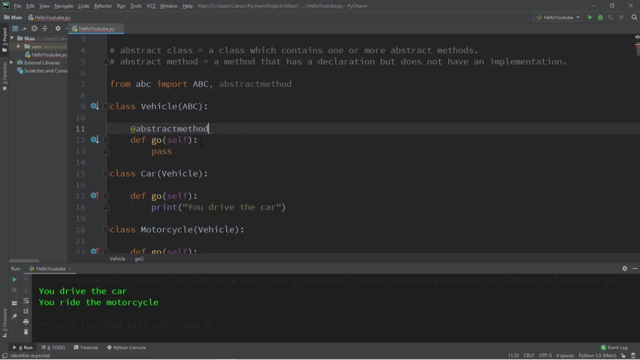 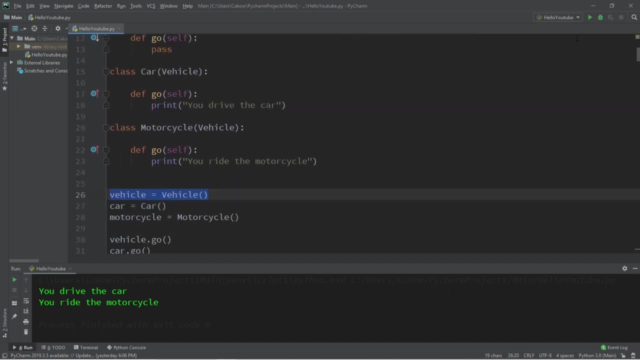 At Abstract Method. Alright, we should now be prevented from creating a Vehicle object. Our Vehicle class is now an Abstract class and we cannot give it a physical form, a physical manifestation. And if we attempt to, you can see here that we have a type error. 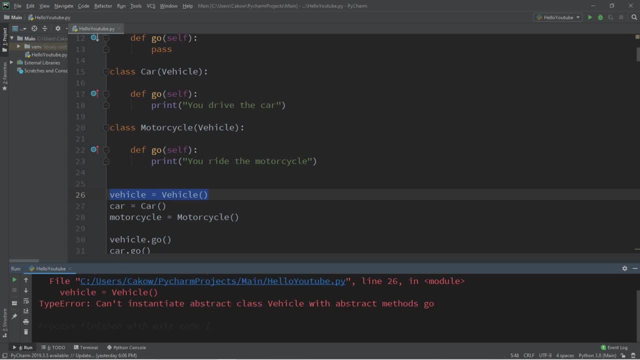 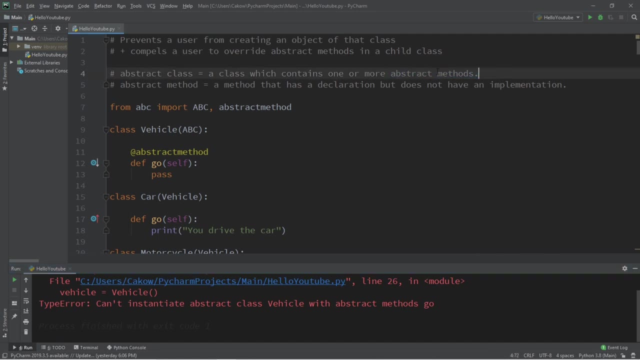 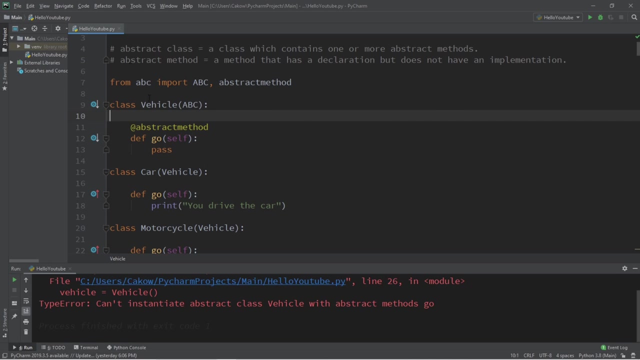 Can't instantiate Abstract class from Vehicle. Vehicle with Abstract methods go. So an Abstract class is a class which contains one or more Abstract methods, And an Abstract method is a method that has a declaration but does not have an implementation. Now, by definition, an Abstract class contains one or more Abstract methods. 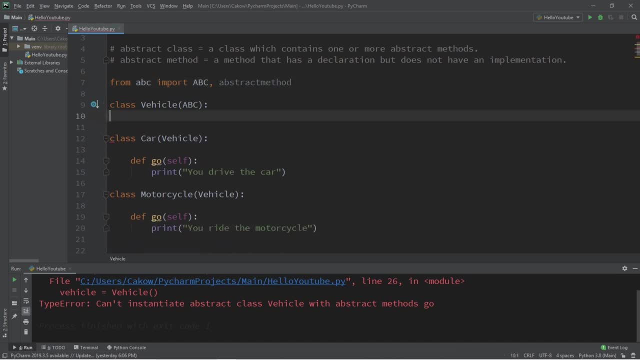 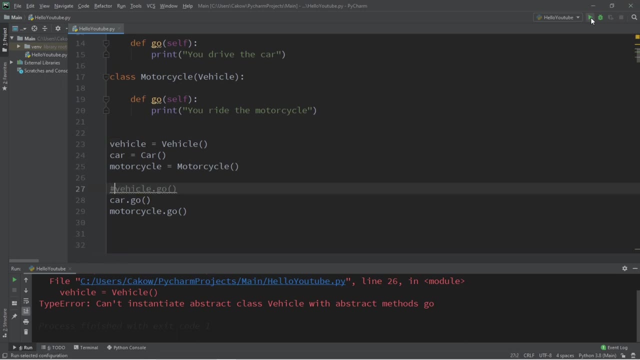 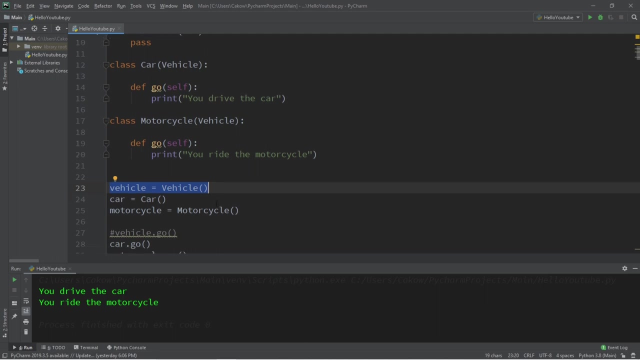 If I remove this one Abstract method within our Vehicle class, well, we could still create a Vehicle object, And I'm just going to turn this Vehiclego line into a comment because we don't have a Go method anymore. As you can see, we can still create a Vehicle object which we would like to prevent a user from doing. 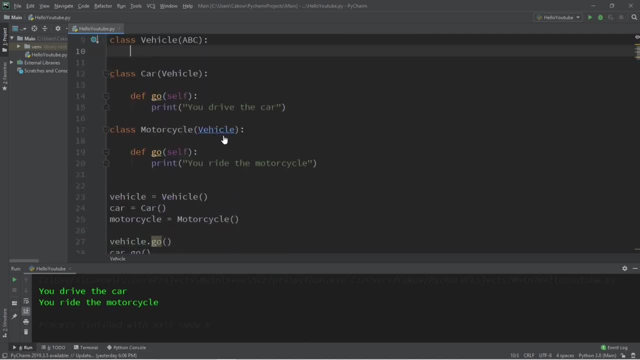 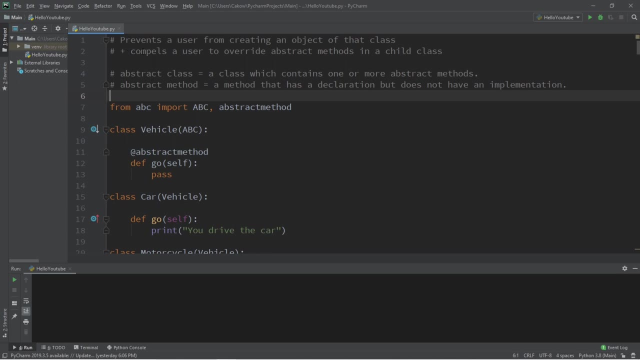 So we need at least one Abstract method within our Vehicle class, So I'm going to go ahead and add this Go method back in. An additional feature of Abstract classes is that they compel a user to override any Abstract methods within a Child class- A method that is Abstract, has a declaration but does not have an implementation. 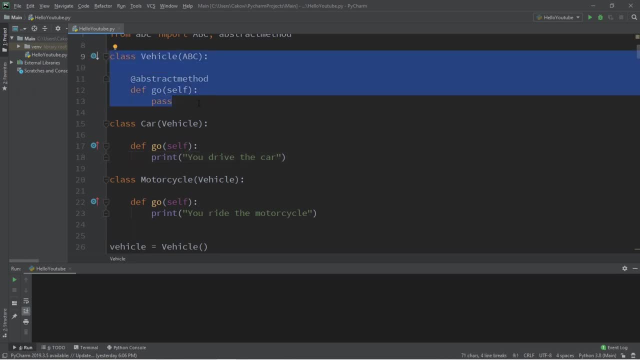 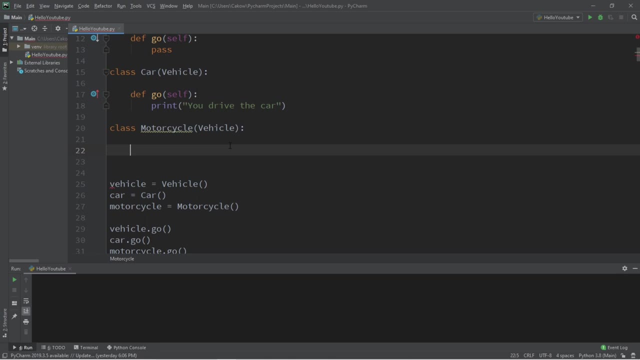 So let's say that we create our Vehicle object, Let's say that we create our abstract Vehicle class, And now we're creating the Children classes of Car and Motorcycle. And let's say I'm not paying attention and I forget to add a Go method. 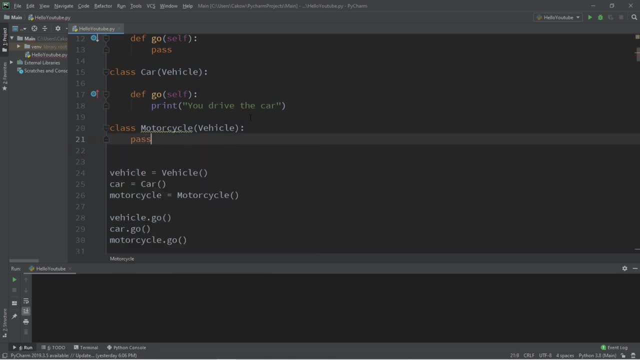 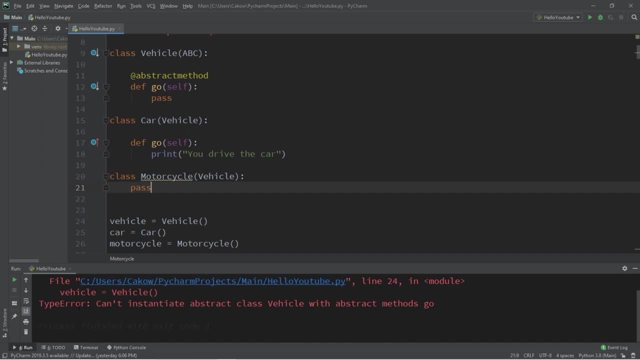 So if I just write Pass within my Motorcycle class, I'm currently missing a Go method within my Motorcycle class. Well, Python is going to prevent me from running this because we have a type error: Can't instantiate Abstract class Vehicle with Abstract methods of Go. 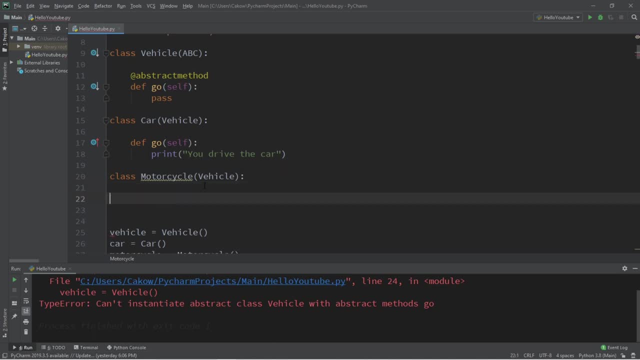 So by inheriting from an Abstract class, it's a good form of checks and balances to be sure that your Children classes are not missing any implementations of any methods that they inherit. Here's an additional way of thinking of this: Our Vehicle class is telling its Children. 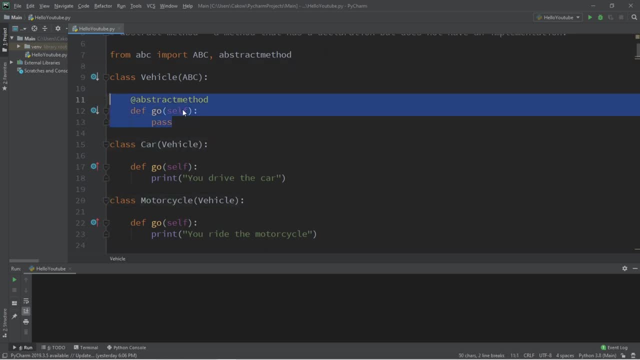 if you're going to inherit from me, then you need to override this Abstract method of mine, And if you don't, well, I'm not going to let you be instantiated. So, in order for us to create a Car and Motorcycle class, 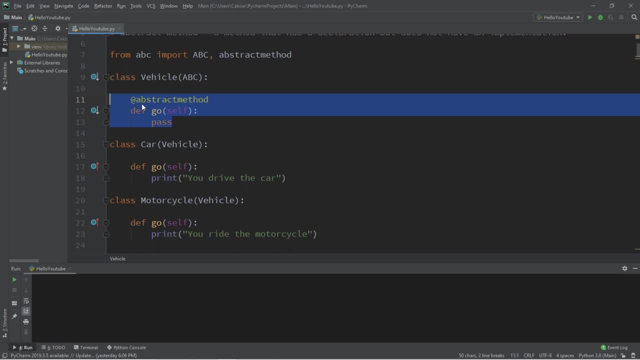 we need to override the Go method that they inherit from its Parent class of Vehicle and provide its own implementation. Now let's say we create an additional method. Let's say we have a Stop method, So let's define that DEF Stop. 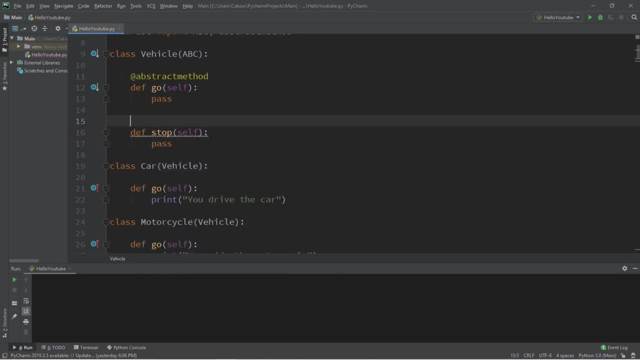 For the time being, I'll write Pass And, to make this an Abstract method, add this decorator At Abstract Method. Now, Car and Motorcycle both need to implement that method of Stop. It's currently missing it, As you can see here. Class Car must implement all Abstract methods. 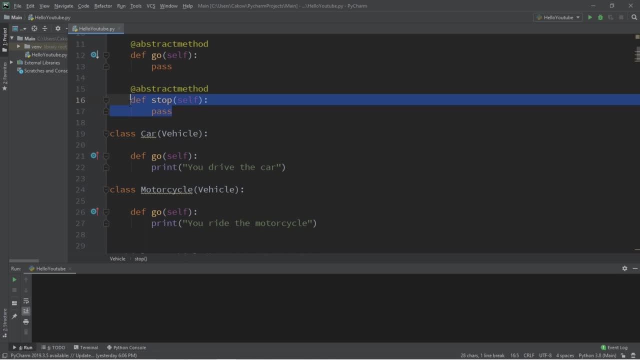 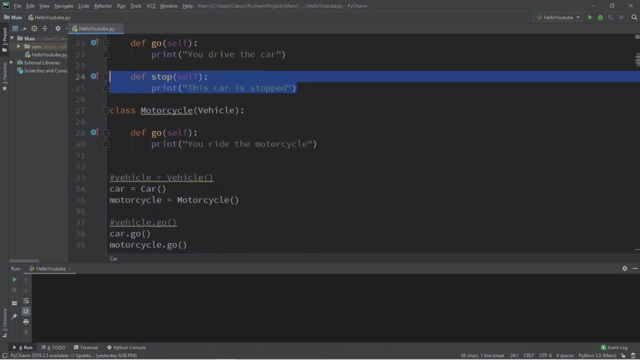 And the same thing applies for Motorcycle as well. So we need to override this method and provide its own implementation. So let's remove that decorator and let's print something. Let's print: This Car is Stopped. And I'll do the same thing for Motorcycle. 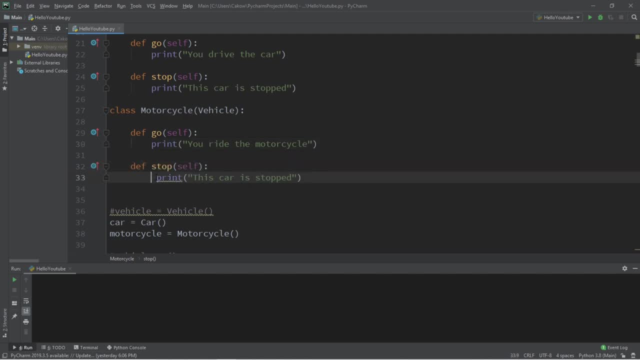 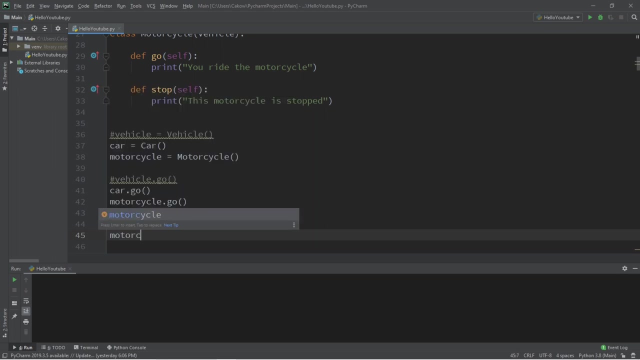 So DEF Stop, Let's say This Motorcycle is Stopped And we'll call the Stop method for each of these types of vehicles CarStop And MotorcycleStop. Alright, and we can now create a Car and Motorcycle object Because we are overriding both of these Abstract methods found within the parent class of Vehicle. 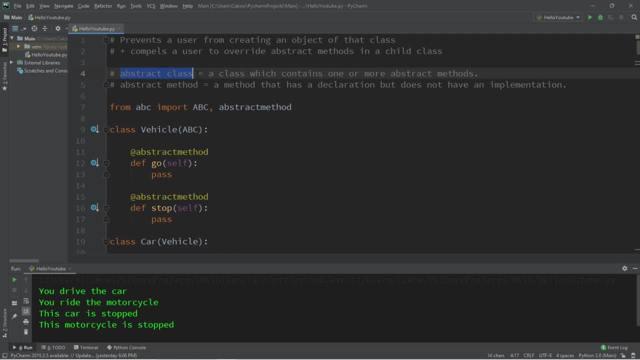 Alright, everybody. so that's the basics of Abstract classes. It's a class which contains one or more Abstract methods, And an Abstract method is a method that has a declaration but does not have an implementation. And the benefits of using an Abstract class. 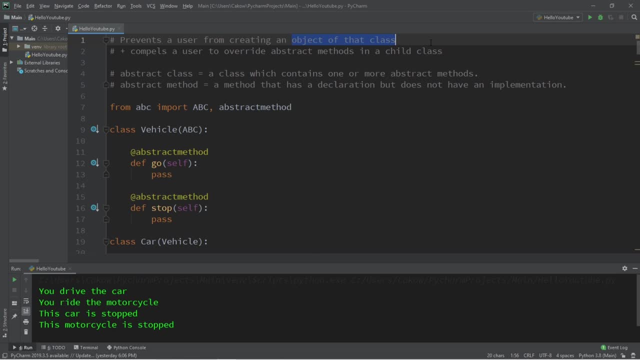 is that they prevent a user from creating an object of that class. Plus, it compels a user to override any Abstract methods found within a child class. So if you would like a copy of this code, I will post all of this in the comments section down below.